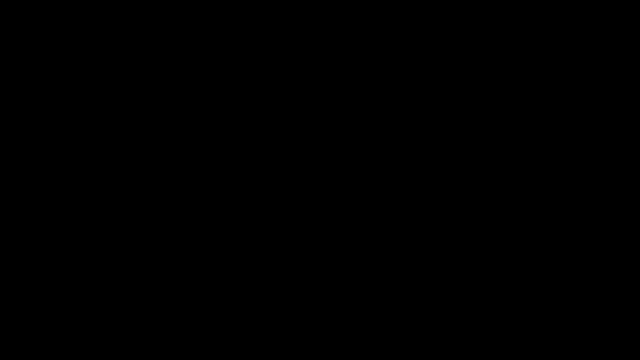 In this video we're going to talk about how to convert a mixed number into a decimal. So the example that I have is 3 and 2 fifths. How can we convert that into a decimal? 3 and 2 fifths is the same as 3 plus 2 over 5.. So all we need to do is 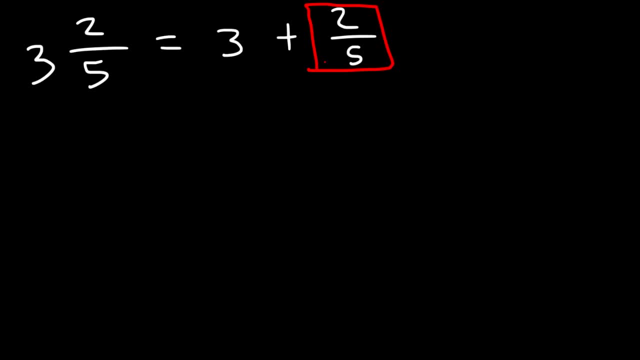 convert this portion of the mixed number into a decimal, And a simple way to do that is to use long division. So 2 over 5 can be expressed this way. Now, how many times does 5 go into 2?? 5 goes into 2 zero times, So we need to add a decimal. 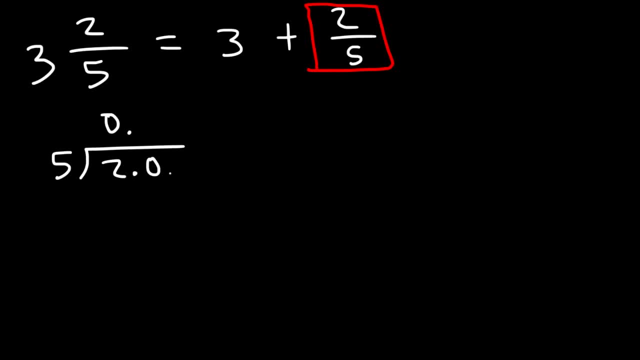 point. Now let's add a zero. Now, how many times does 5 go into 20?? 5 goes into 20 four times. So 5 go into 2, 0.4 times. 5 times 0.4 is 2.. 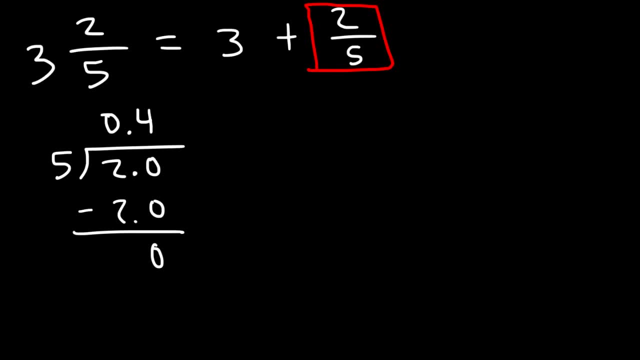 So 5 goes into 2 0.4 times. So 5 goes into 2 0.4 times. 5 times 0.4 is 2.. So if we subtract 2 minus 2, we get 0.. So this means that 2 over 5 is equal to what? 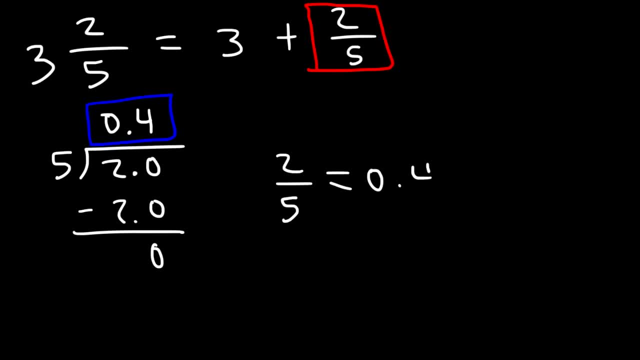 we see here, and that is 0.4.. So this is 3 plus 0.4, which is 3.4.. And so that's how you can convert a mixed number into a decimal. But for the sake of practice, let's go ahead and work on a few more examples. 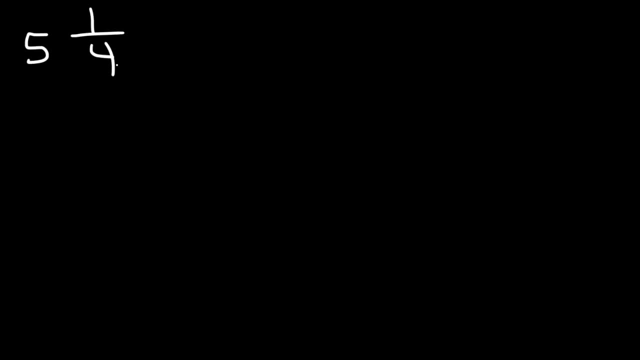 Try this one: 5 and 1. fourth, Go ahead and convert it into a decimal, So this is going to be 5 plus 1 over 4.. And, just like before, we're going to focus on that fraction, So let's use long division. 4 goes into 1 zero times, So we need to. 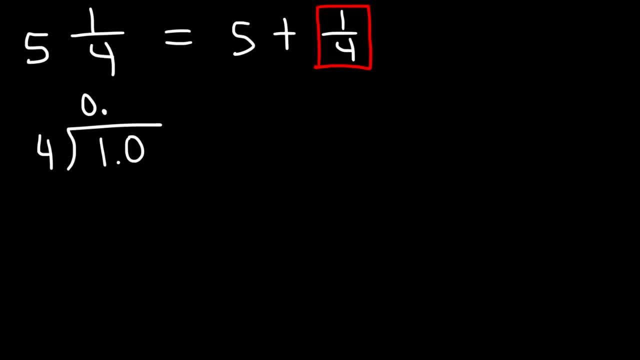 add a decimal Now, how many times does 4 go into 10?? 4 goes into 10 2 times. 4 times 2 is 8.. So 4 times 0.2 must be 0.8.. 1 minus 0.8 is 0.2.. So we're. 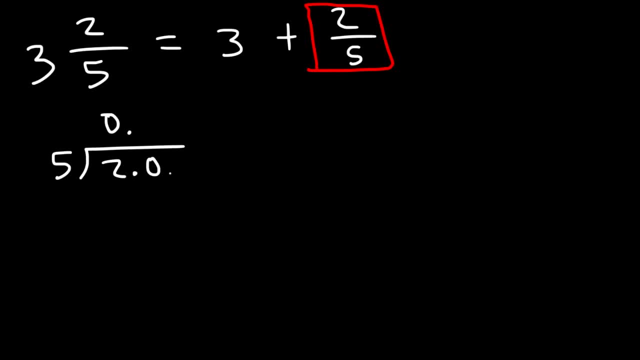 point. Now let's add a zero. Now, how many times does 5 go into 20?? 5 goes into 20 four times. So 5 go into 2, 0.4 times. 5 times 0.4 is 2.. 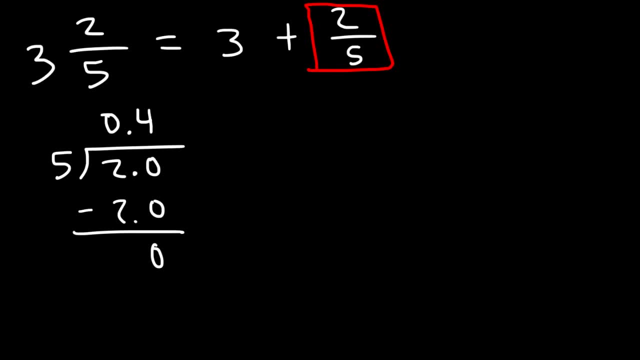 So 5 goes into 2 0.4 times. So 5 goes into 2 0.4 times. 5 times 0.4 is 2.. So if we subtract 2 minus 2, we get 0.. So this means that 2 over 5 is equal to what? 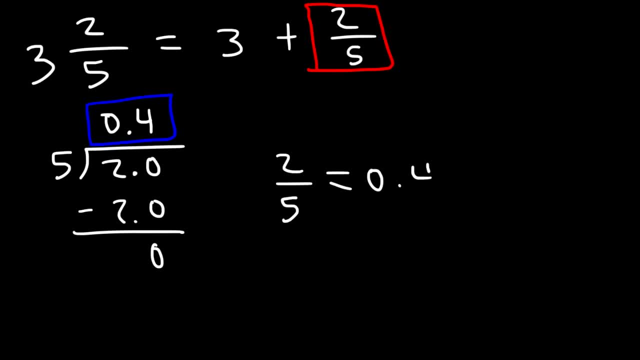 we see here, and that is 0.4.. So this is 3 plus 0.4, which is 3.4.. And so that's how you can convert a mixed number into a decimal. But for the sake of practice, let's go ahead and work on a few more examples. 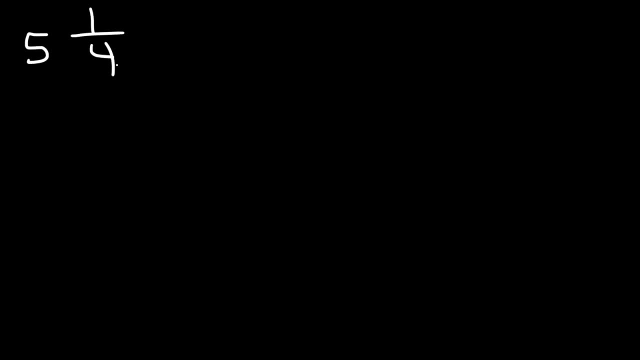 Try this one: 5 and 1: 4. Go ahead and convert it into a decimal, So this is going to be 5 plus 1 over 4.. And, just like before, we're going to focus on that fraction, So let's use long division. 4 goes into 1, zero times, So we: 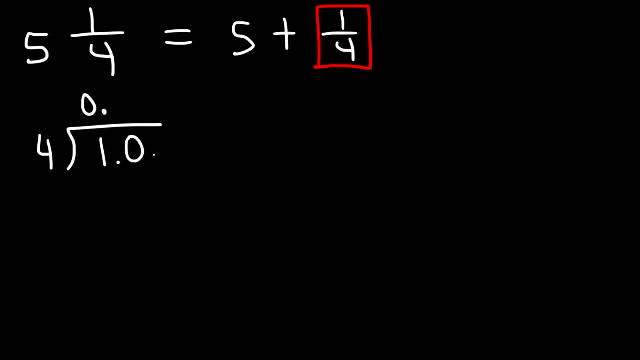 need to add a decimal. Now, how many times does 4 go into 10?? 4 goes into to 10 two times. 4 times 2 is 8, so 4 times 0.2 must be 0.8.. 1 minus 0.8 is 0.2.. So we're. 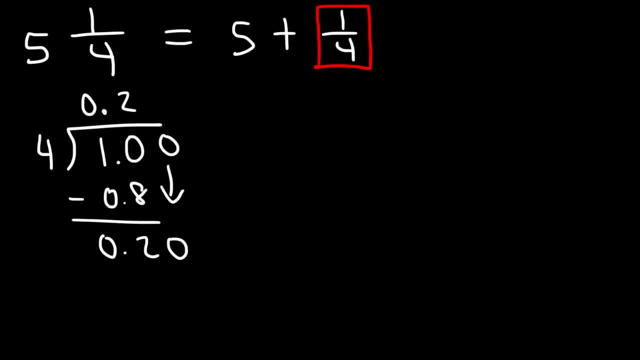 going to add a 0 and treat 0.20 as if it's 20.. 4 goes into 20 five times. So we're going to get a 0 now. So we could say that 1 over 4 is equal to 0.25.. So 5 plus 1. fourth is: 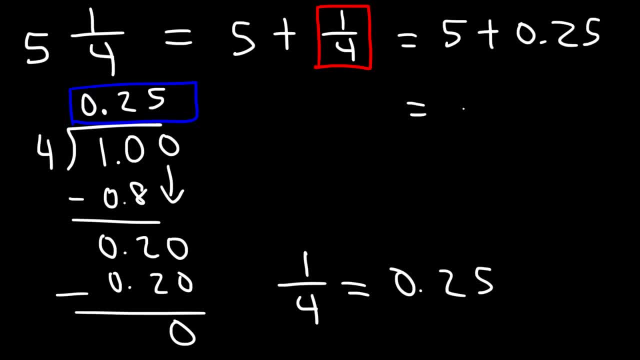 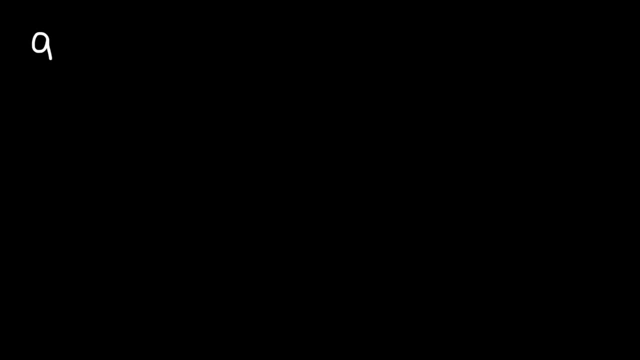 5 plus 0.25, which is 5.25.. And so that is the value of this mixed number. 5 and 1, fourth, is equal to 5.25.. Now let's move on to our third example: 9 and 7 eighths. Feel free to pause the video if you want to try this problem. 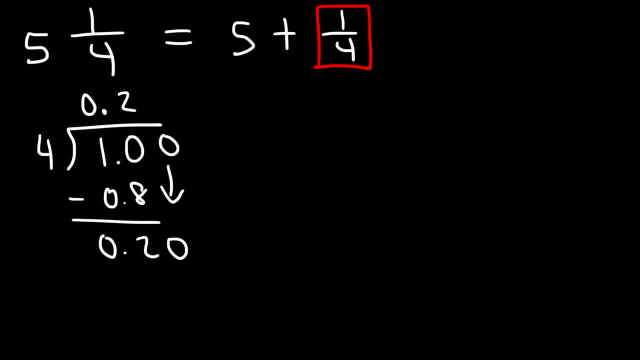 going to add a 0 and treat 0.20 as if it's 20.. 4 goes into 20 5 times, So we're going to get a 0 now, So we could say that 1 over 4 is equal to 0.25. 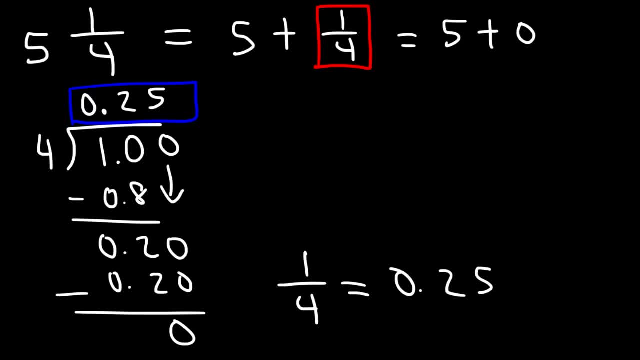 So 5 plus 1. fourth is 5 plus 0.25.. Which is your final m tense in this case, And so that is the value of this mixed number. 5 and 1. fourth is equal to 0.25.. 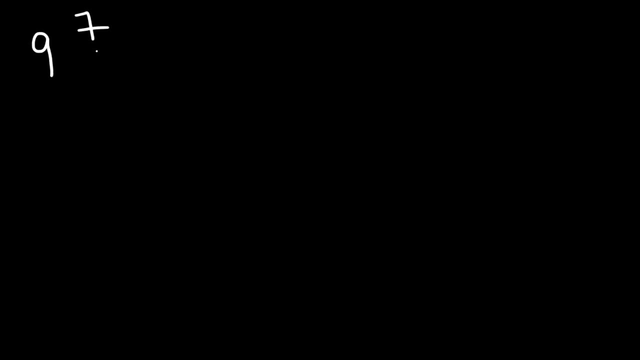 Now let's move on to our third example: 9 and 7 eighths. Feel free to pause the video if you want to try this problem. So this is gonna be 9 and 7 eighths plus seven over eight, and we need to focus on converting this fraction into a. 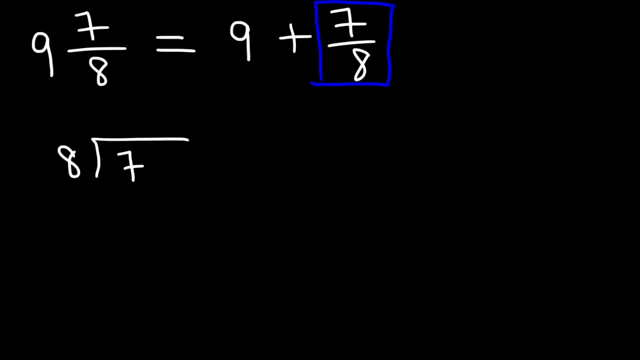 decimal. so eight goes into seven, zero times. now how many times this eight go into seventy eight times eight is 64. 8 times 9 is 72 and 72 exceeds 70. so we could say 8 goes into 78 times 8 times 8 is 64. so 8 times 0.8 is 6.4, 7. 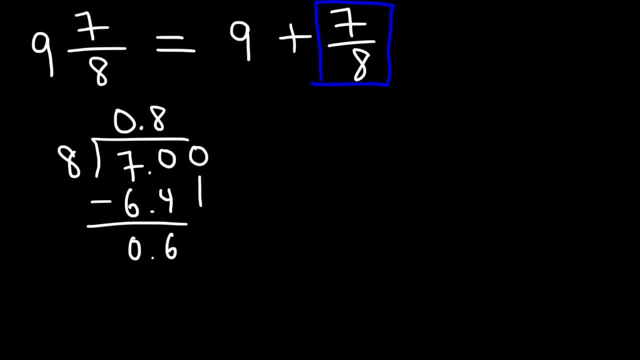 minus 6.4 is 0.6, and so let's bring down to 0. now how many times this 8 go into 60? 8 goes into 60. 7 times 8 times 7 is 56. 60 minus 56 is 4. so if we add a 0 and get 40, 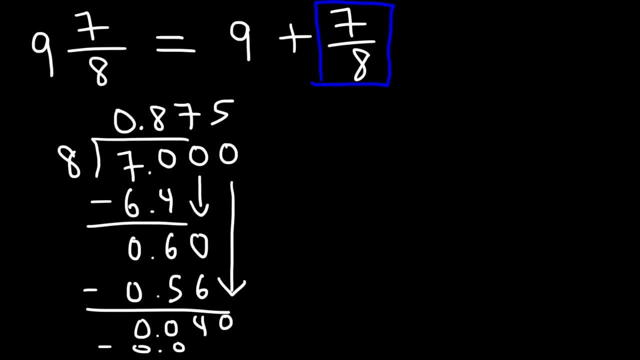 8 goes into forty five times, and so at this point we're going to get a remainder of zero, and so we could say that seven over eight is equal to the result that we see here, and that is point eight, seven five. so this is nine plus point eight, seven five, and so that's nine, point eight, seven, five. thus, 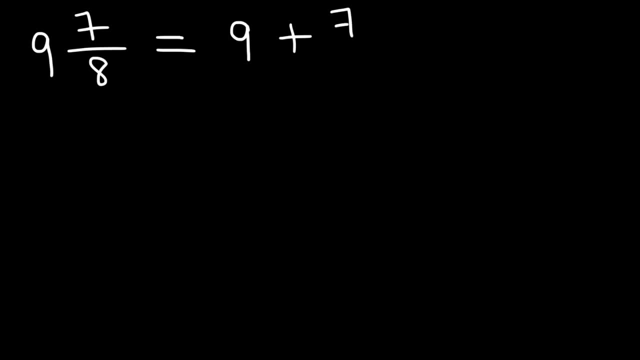 So this is going to be 9 plus 7 over 8.. And we need to focus on converting this fraction into a decimal. So 8 goes into 7, zero times. Now, how many times does 8 go into 70?? 8 times 8 is 64.. 8 times 9 is 72.. And 72 exceeds 70. So we could say 8 goes into 70. 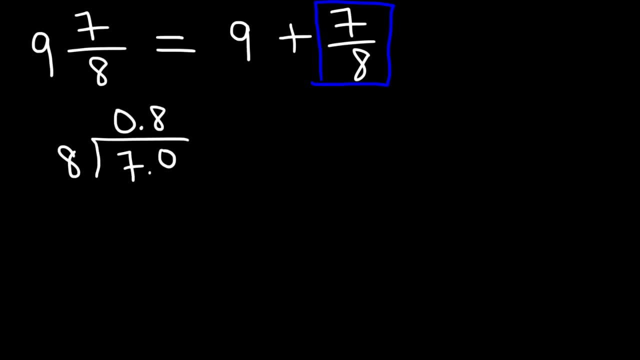 8 times 8 times 8 is 64.. So 8 times 0.8 is 6.4.. 7 minus 6.4 is 0.6.. And so let's bring down the 0.. Now, how many times does 8 go into 60?? 8 goes into 60. seven times 8 times 7. 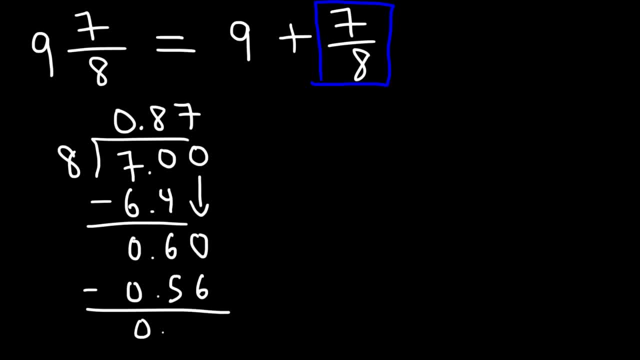 is 8.. That's 10.. So 8 times 7 minus 6 is 56.. 6d minus 66 is 4.. So if we add a zero and get 40,, 8 goes into 40 extant five times, And so at this point we're going to get a. 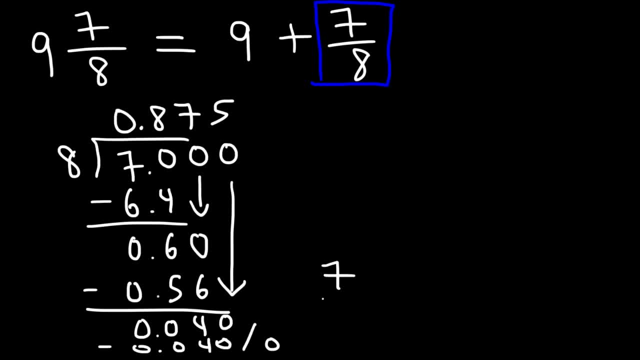 remainder of zero, And so we could say that 7 over 8 is equal to the result that we see here, and that is .875.So this is 9 plus .875. And we're going to add 8. Here's an example. 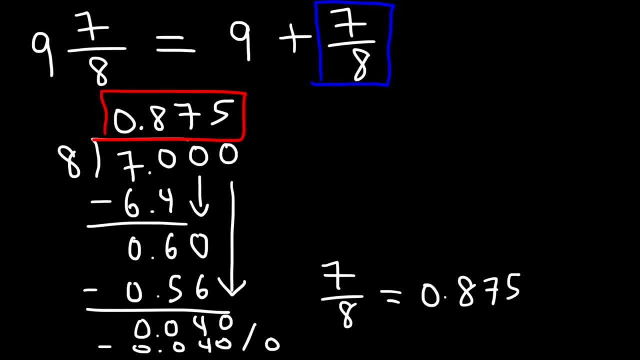 Let's just say 9 plus 8 plus 3 is 8.. So here what the second four is making. See, this is an example of how we can get into that other airplane triangle Here. in our last example we start atboyscom Fourth is 4 passed by his answer. so this is called abnormal этих. 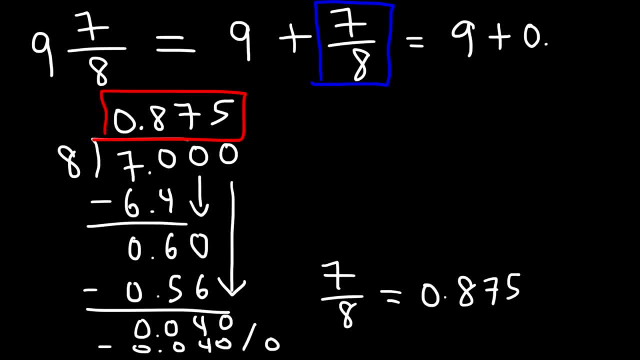 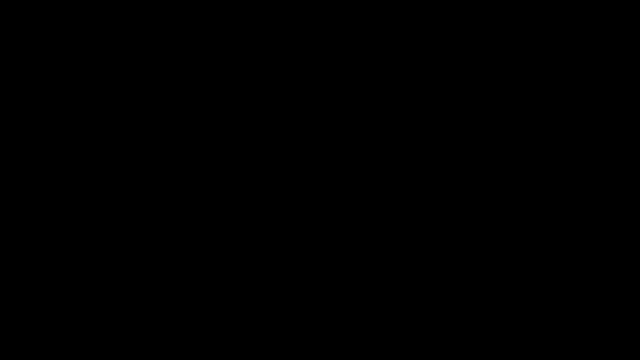 tarte or critical 상태 line law. So first we are going to find the negative. So this is 9 plus .875, and so that's 9.875.. Thus that is the value of this mixed number. 9 and 7 eighths is 9.875.. 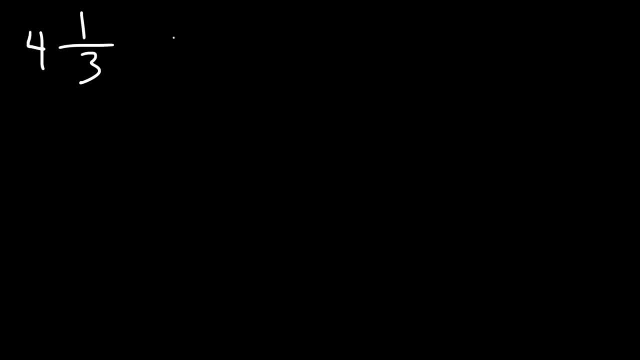 Let's work on one more example: 4 and 1 third. Pause the video and work on it. So this is going to be 4 plus 1 third. So let's convert 1 over 3 into a decimal. 3 goes into 1 zero times. 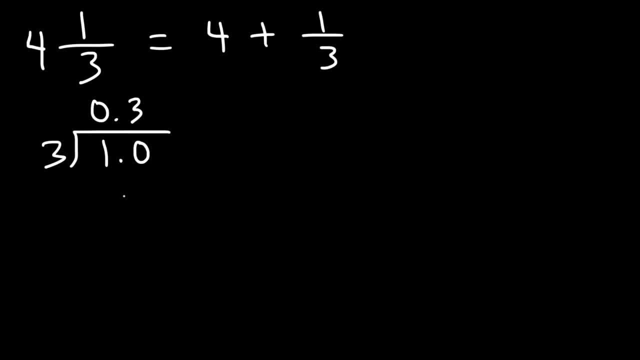 3 goes into 10 three times. 3 times 3 is 9, so 3 times 0.3 is 0.9.. 1 minus 0.9 is 0.1.. If we add a 0,, 3 goes into 10 three times.